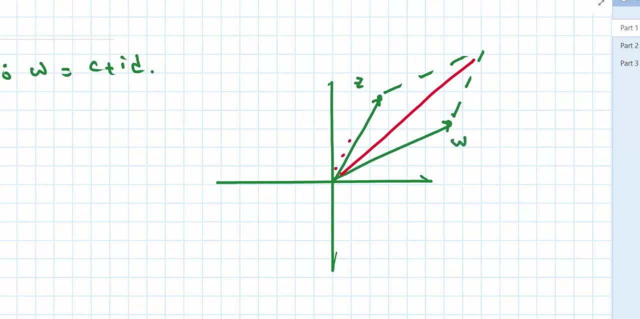 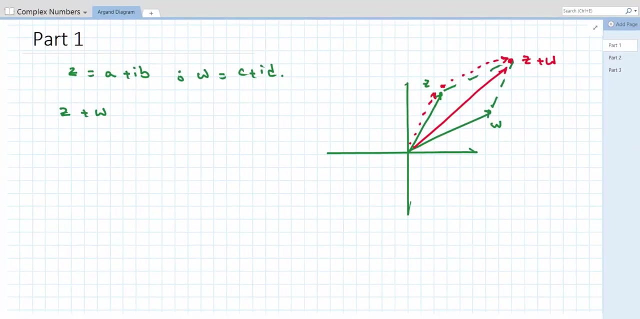 Then what's happening is we're starting with z, heading up to here and then adding w, so the tail of w sits at the head of z and then the vector is drawn and wherever we end up with is the new vector z plus w. So if we have a look at algebraically what that means, 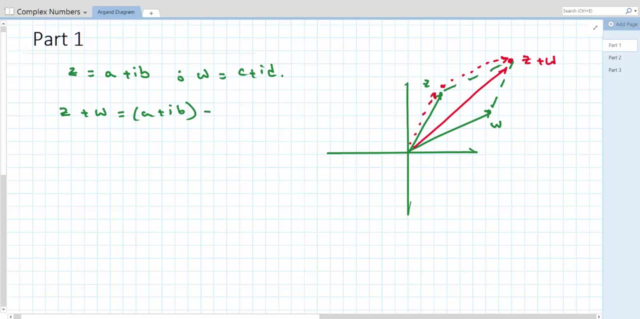 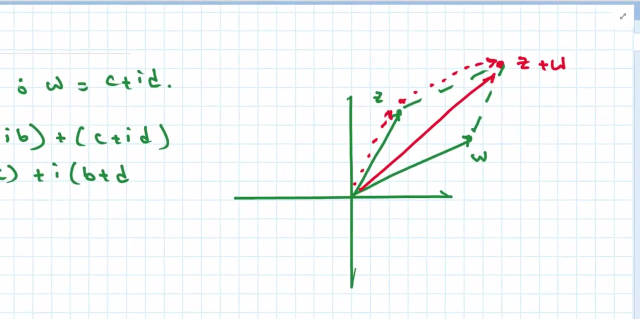 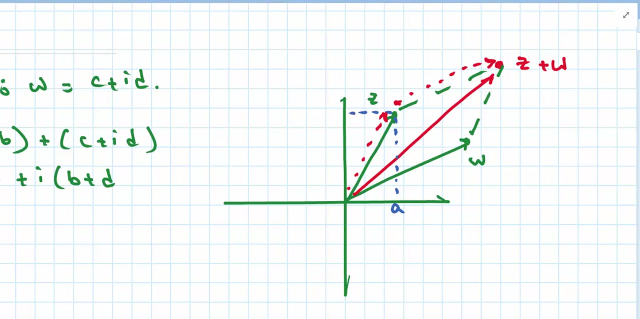 That's a plus ib, plus c plus id. The real part is a plus c and the imaginary part is b plus d. Now let's look at what's happened on our vector diagram. That would be a, This would be b, Here's c. 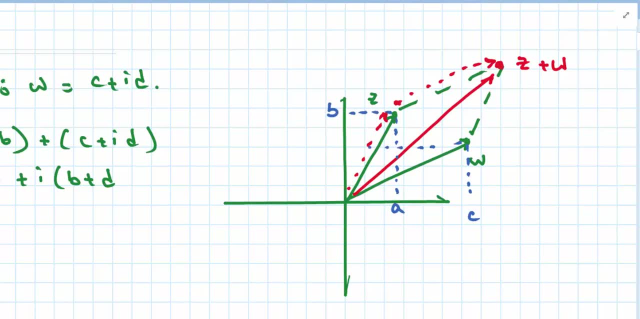 This would be a, This would be b, Here's c, Here's d And here's d. When I add these two vectors, c and a get added together, So the resultant is a plus c, And my diagram's not quite perfect, but you can see what's happening. 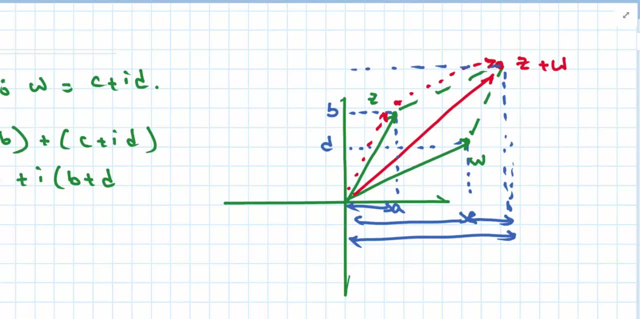 And then the same is true for the imaginary, The imaginary part of the addition where we're adding a, b and d, so that d gets added on top b plus d, resulting in the new position When we do a vector addition. then we're just taking the real values of a and b. 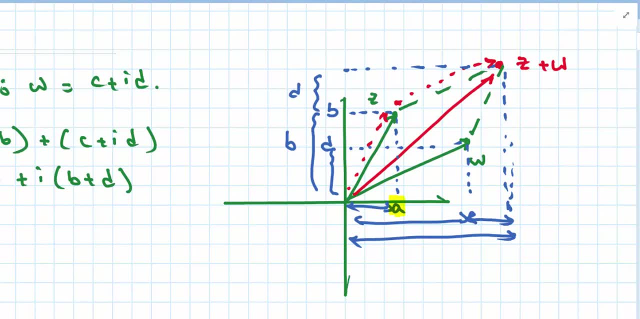 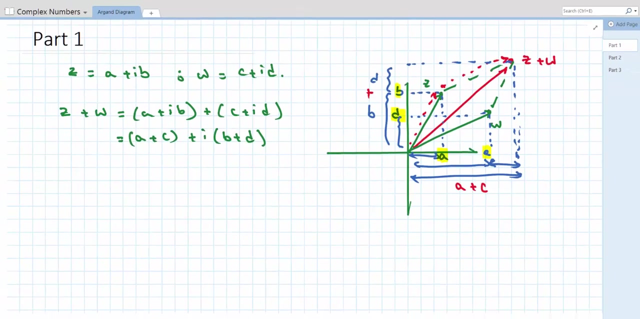 And c, which I've lost here, And we're adding those two together, And we're taking b and d and we're adding them together to find the position of the new vector. So that's addition. What about subtraction? Now, subtraction seems a bit more, a bit confusing. 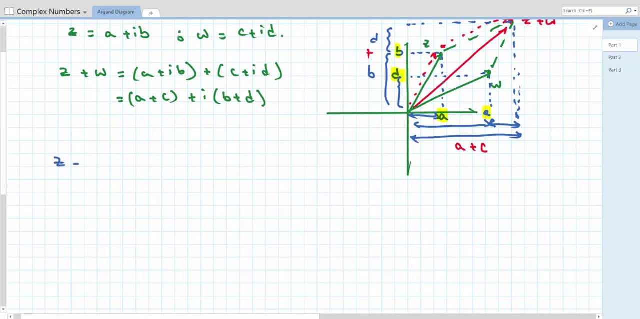 But if we go back to our algebraic format of how this works, then you can see that we'll end up with a minus c plus i, b minus d. So what we're doing is taking the new position And what we're doing is taking the real value of the second vector away from the real value. 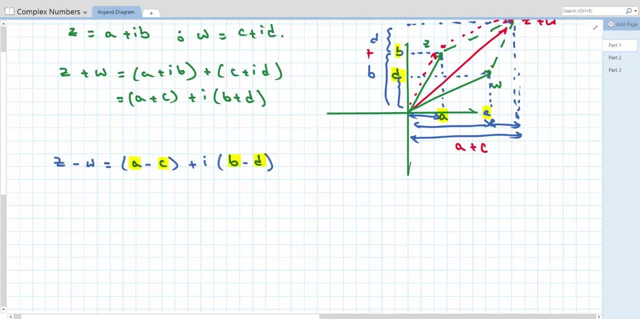 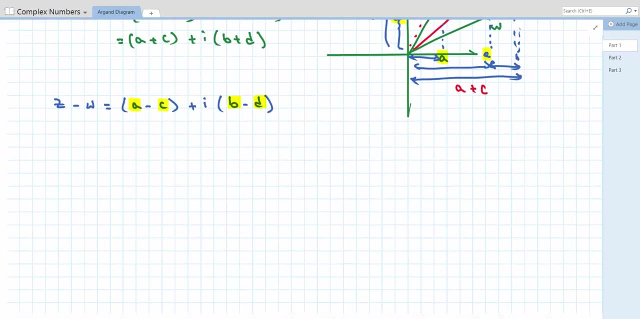 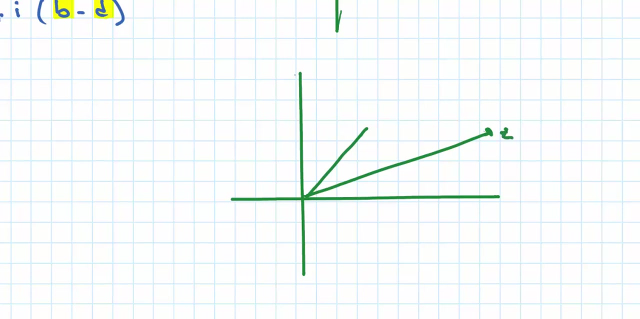 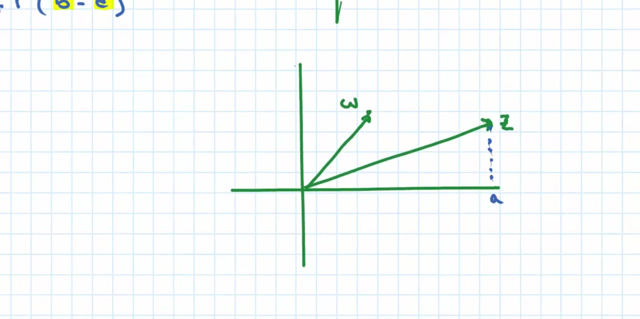 of the first And similarly the imaginary parts are being subtracted. So how does that look on a vector diagram, on an argon diagram? So this time I am going to set this as my z, And here's my w. That would be a. 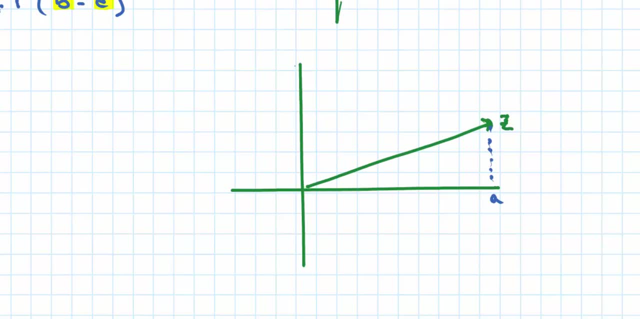 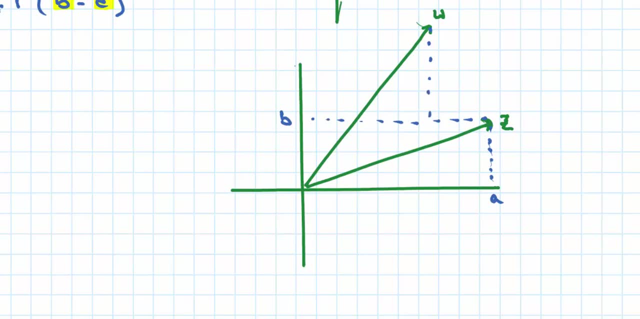 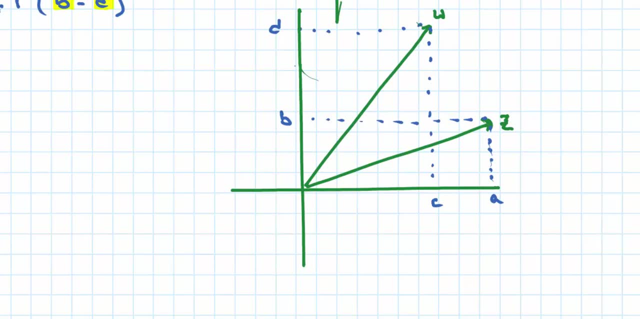 Okay, So we are subtracting c from a, So that would leave me with Point along here. Maybe that's not the most accurate. Let's see: Here is c And I am subtracting a amount from it, So we are going back a amount. 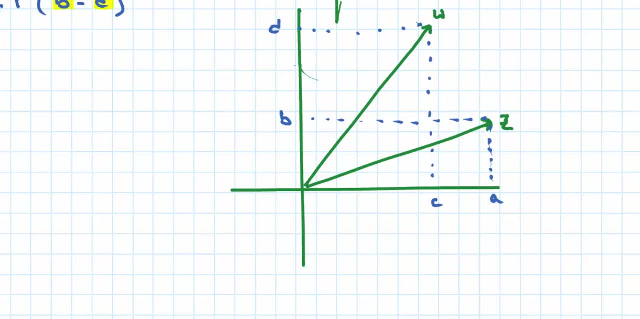 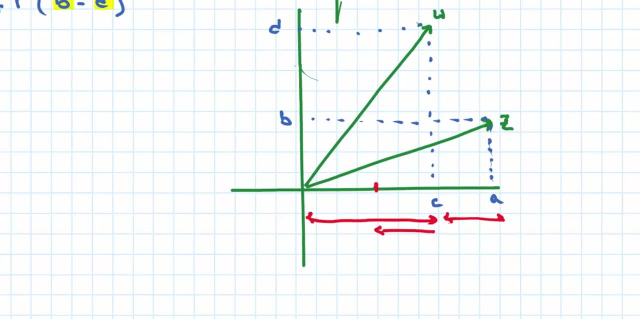